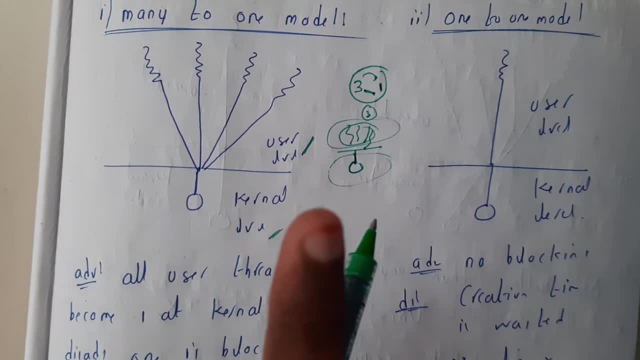 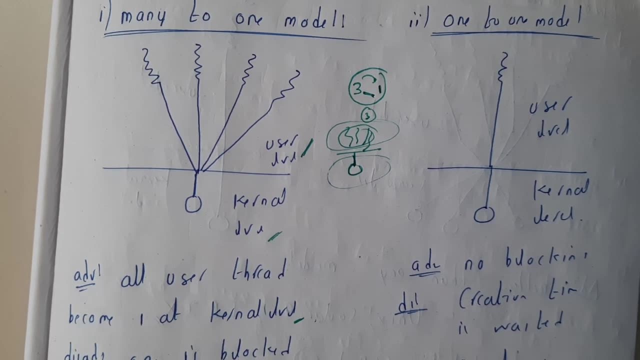 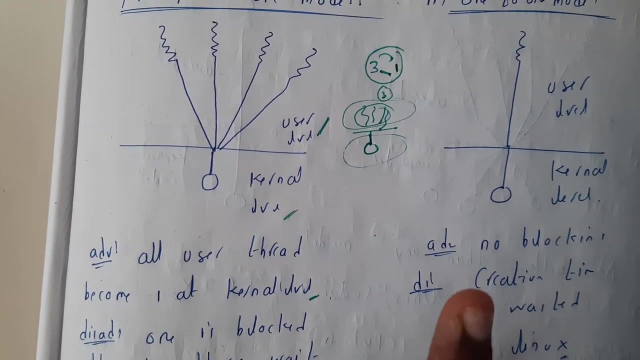 be the advantages in this situation? All user threads become one at the kernel. So that's an advantage, basically, but it is also an disadvantage, Right? I hope everyone got a small idea on this, Okay. So what will be the disadvantage guys? So what if one thread is blocked? What will be the situation? So let us assume this. 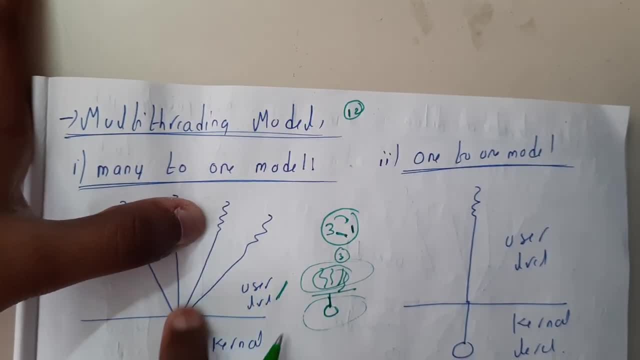 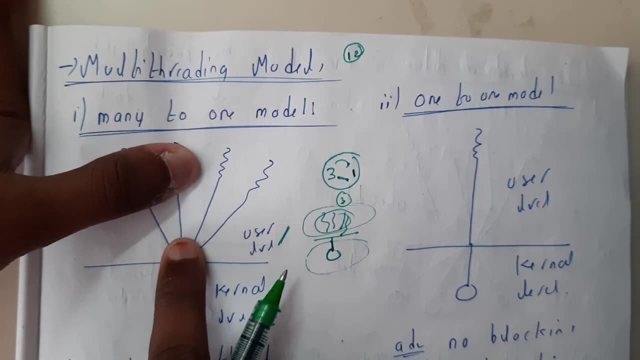 thread is blocked. This thread execution is done. This thread is blocked, So there is no chance of going to the next thread because there is only one kernel. So it is going to wait here, only It is blocked. What should I do? It is blocked. What should I do? Like. 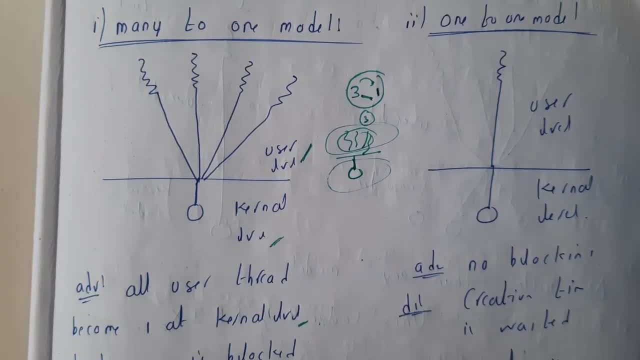 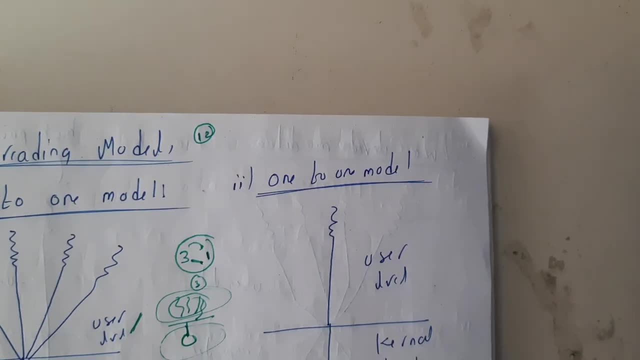 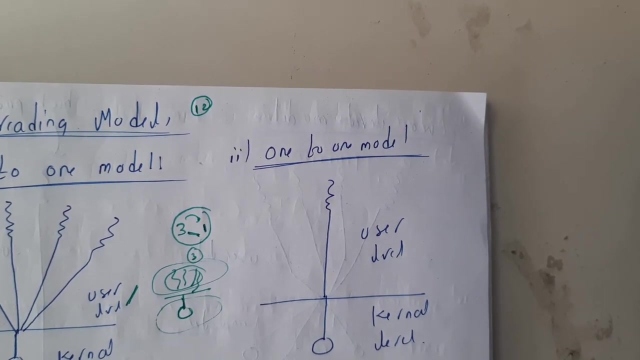 that it's going to just go into that problem. So one is blocked, then all others need to discard. So that will be an issue. Further, moving on the second type, The second type is one-to-one model, So from the name we can again say it is one-to-one. 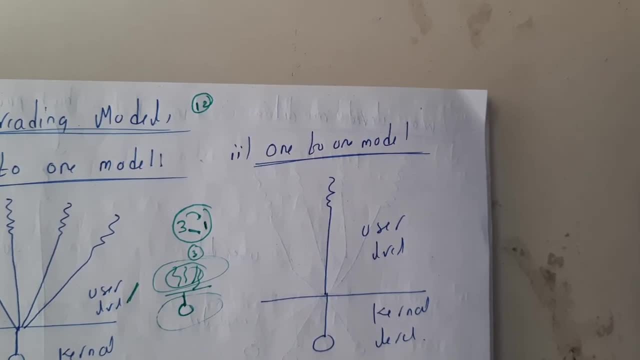 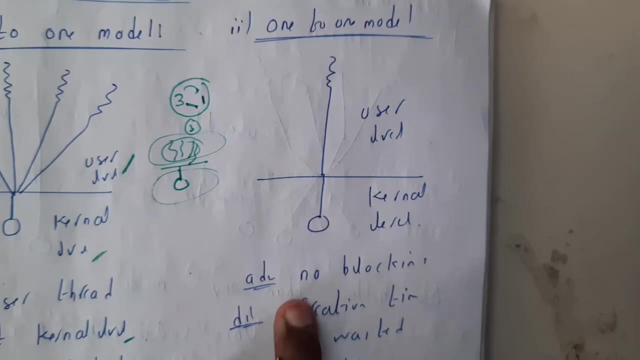 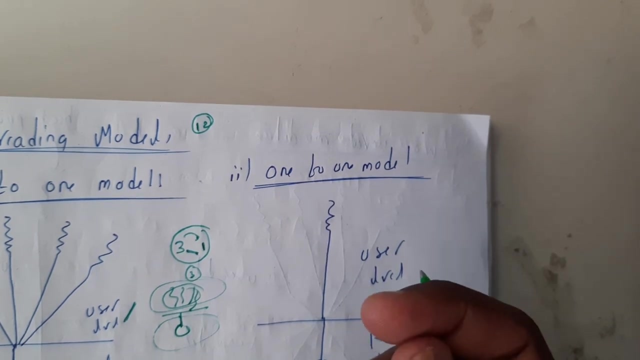 Only a single user. sorry, single user level thread becomes a single kernel level thread, guys. So basically, here the advantage will be: there is no chance of blocking, But the disadvantage is for every small process. Yes, I am asking you. Maybe you don't know what we are going to call bes庇ketia 가. 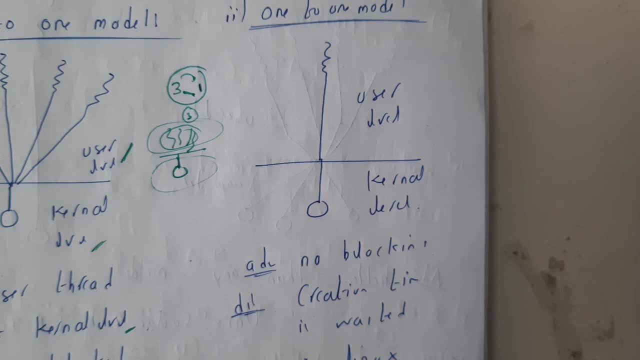 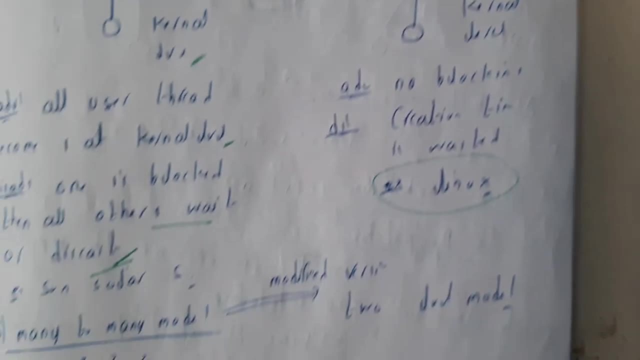 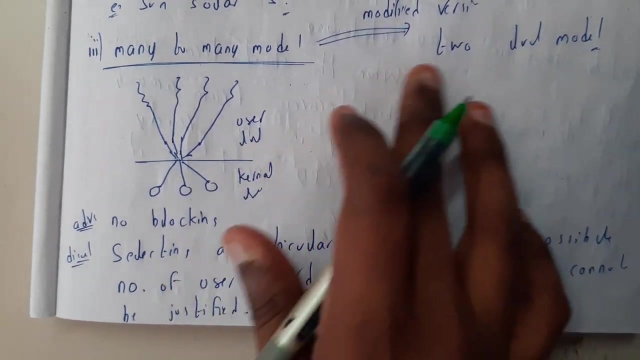 every small thread you need to create as individual, you need to allocate the kernel separately. so that could be an issue. but this is being followed in linux, fine. so now the latest thing, or the third thing with it is nothing but many to many model. so this modified version is two level model. this 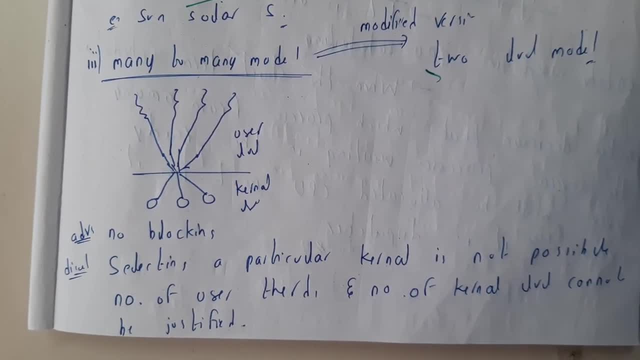 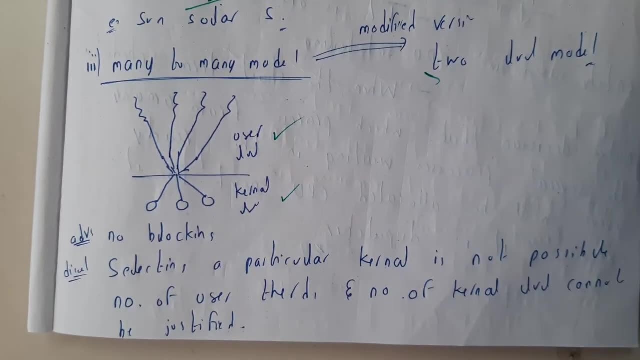 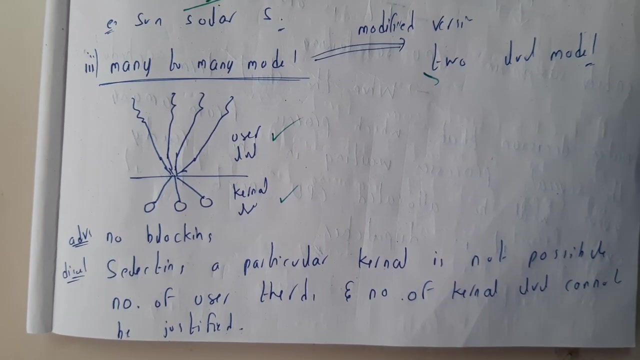 is currently being in use, guys, so many to many- mode, so this is nothing but many to many. so here there will be many user level threads, and below also you will be having many kernels. so fine, so what will be the advantage? so here also, there is no chance of blocking because we are having 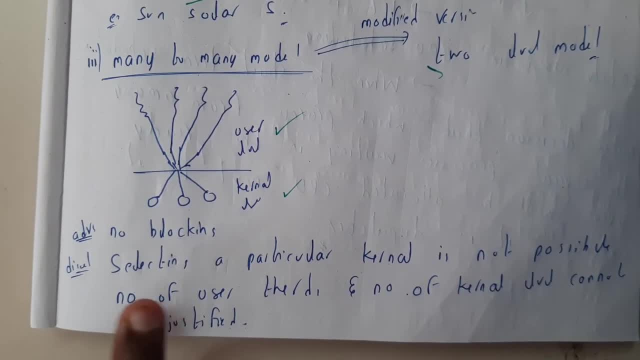 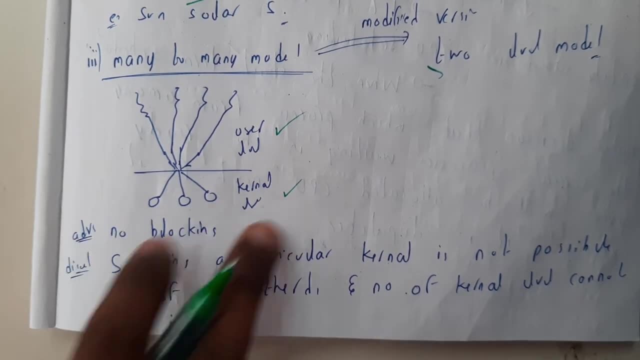 more kernels than many to one so. but the problem will be selecting a particular kernel is not possible. so let us assume this guy wants to take which kernel. so that's an issue. right, we need to select it. the process need to select him. selecting by us is really simple, but the process should know. 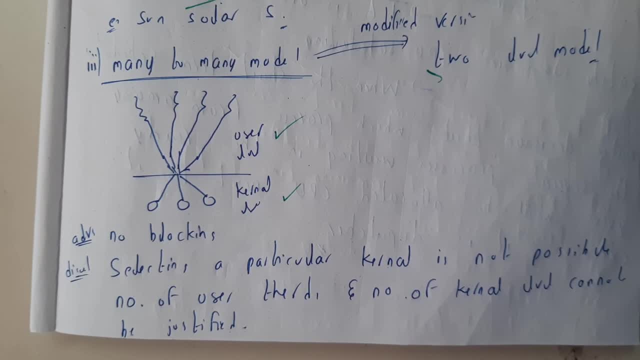 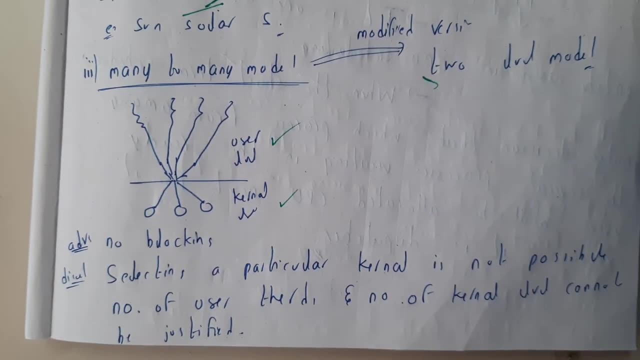 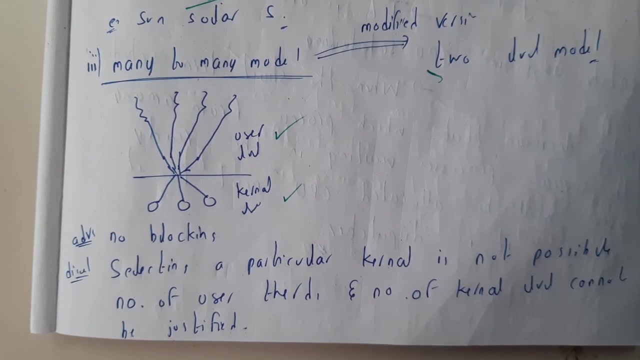 what to select and if it's already like it should wait. so those will be the issues. and even there is one more problem: that we should have an idea about how many threads and how many kernels should be there. so number of user threads and number of kernel levels cannot be justified. so that will be a major issue with this, so that